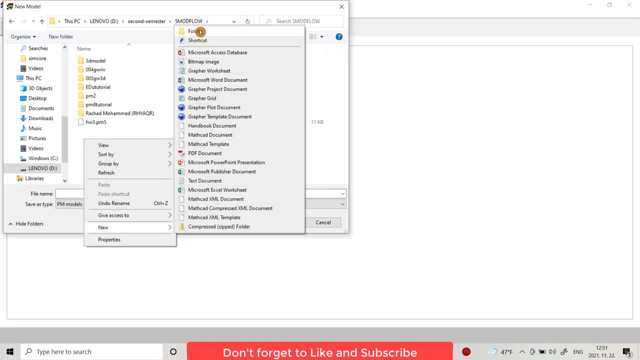 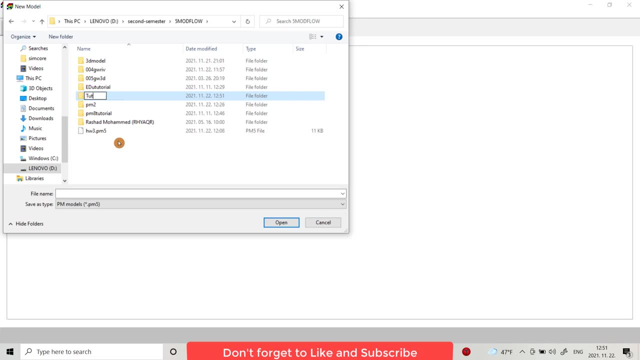 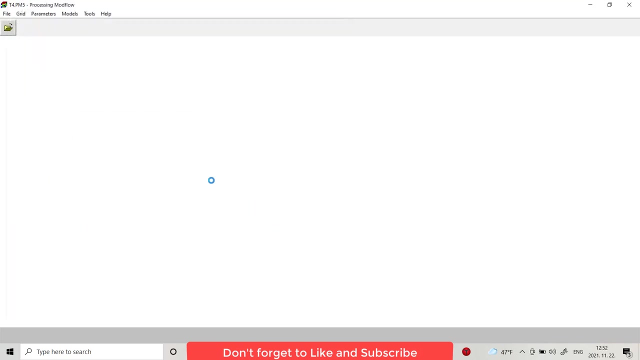 For example, I provide a folder: tutorial4 and tutorial4, ok, Save. Regarding the third tutorial, I have a tutorial I published before. You can use it as a third one. I put the link for all previous tutorials in the description. You can find it easily. 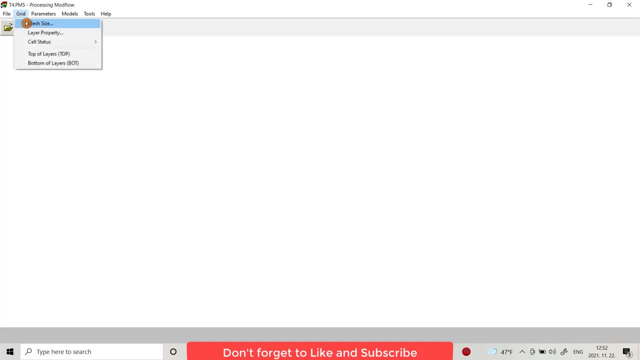 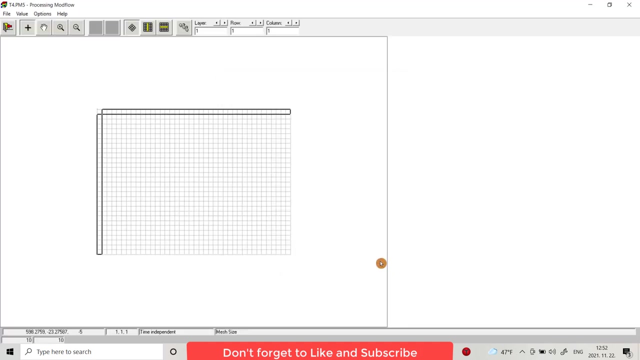 Paste Grid Mesh. I want to have two layers Also, x-axis 30 row, Y-axis 30 row and 300 meter. Regarding x-axis, I want 40 column and 400 meter. Ok, Yes, To be. 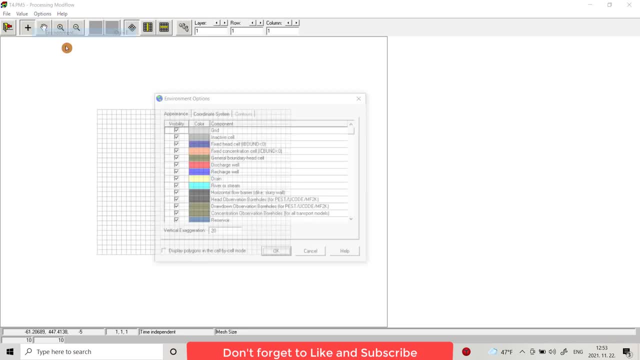 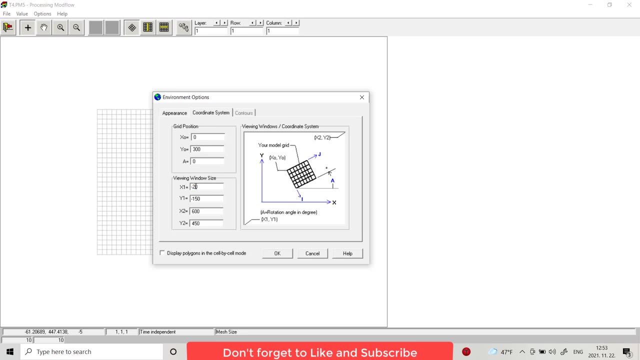 appear better from option environment coordinate system. I want 20, minus 20, x1 and minus 20, y1.. 400, we have x400,, so I want appear till 420.. And y300, I want appear, or the y-axis 320.. 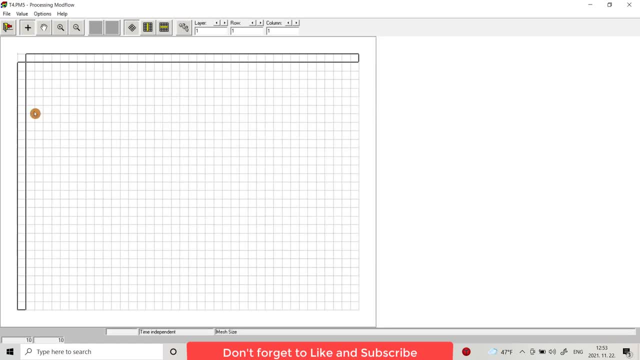 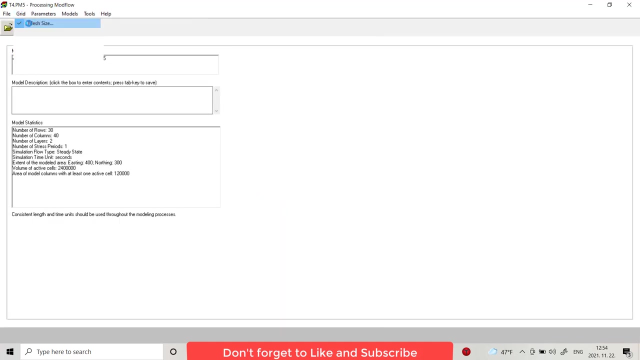 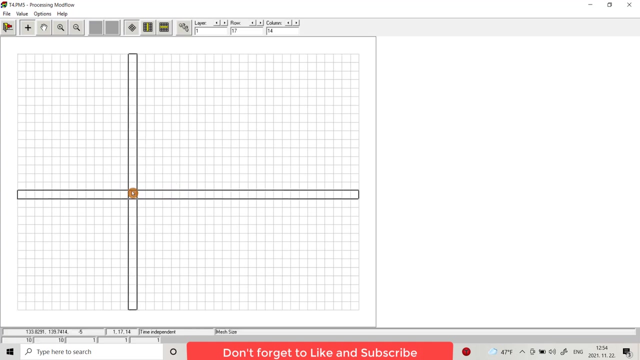 As you see Here, minus this corner is minus 20 to minus 20, if x here 420 to 320.. Coordinate Ok, Save. Yes. Also, I want make it refinement, Make it active here, Yes. 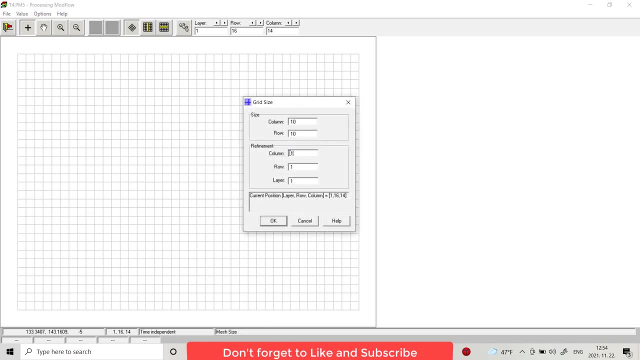 Here I choose this one And make refinement. I want 3 column and 3 row, Ok, Then you can copy To here. Here also, Also, you can copy To here. That's the location of wireless. Now it's good. 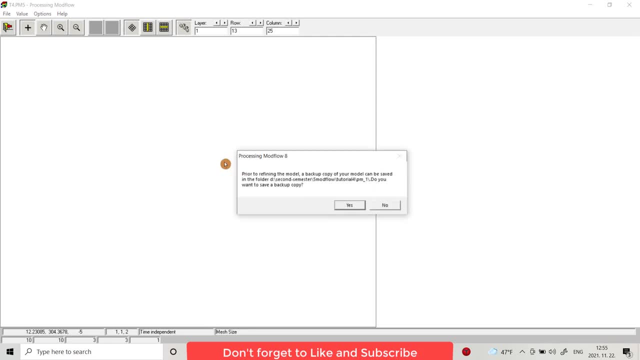 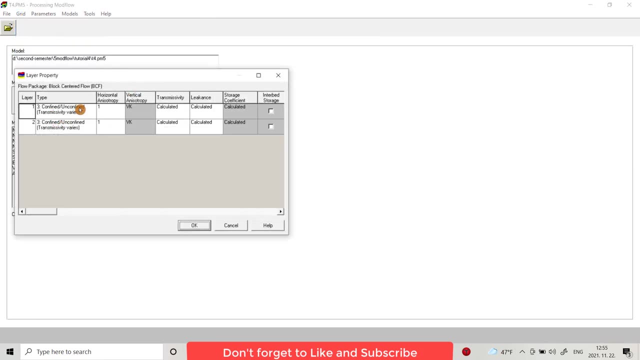 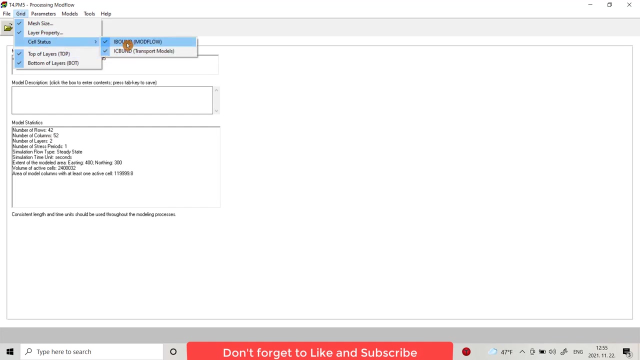 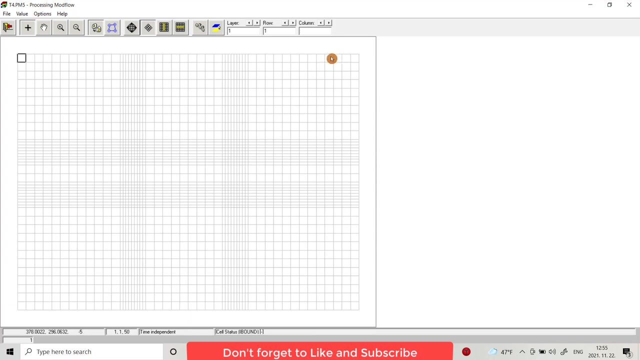 Yes, Yes, save. Ok. Layer properties: Confined and confined. Confined and confined transmissivity. confined and confined transmissivity varies. this one is good for all cases. i choose this one. yes, okay, regarding cell status, i change. uh, this hydro is a hydraulic. for this boundary layers constant make by provide minus. 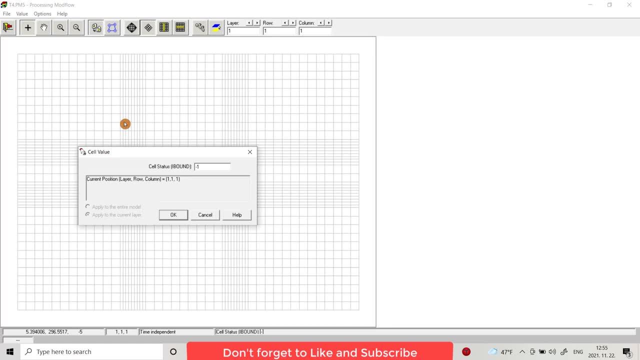 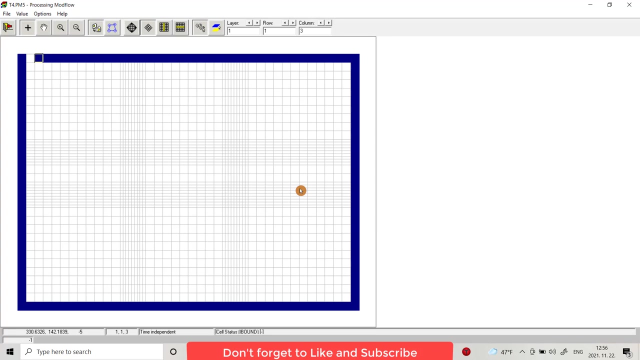 one. one is the body. zero, it will be inactive. minus one, it will be constant. i choose minus one. then copy, and by arrow in your keyboard you can go down. okay, yes, and provide for both layers by this um tool, this one- and go to second layer. it provide for the second layer also, yes. 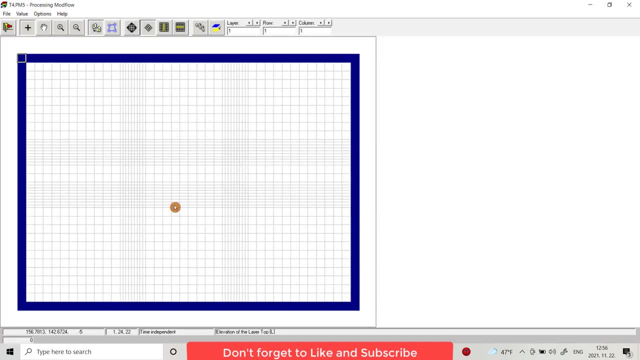 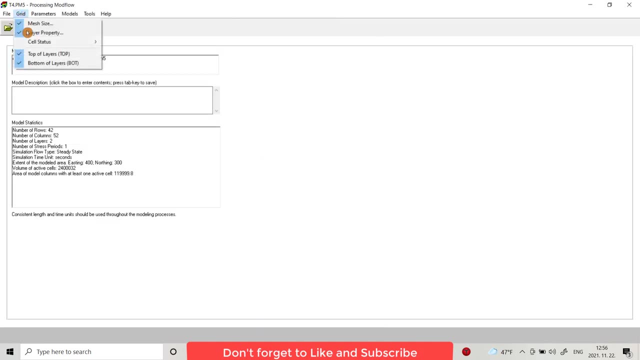 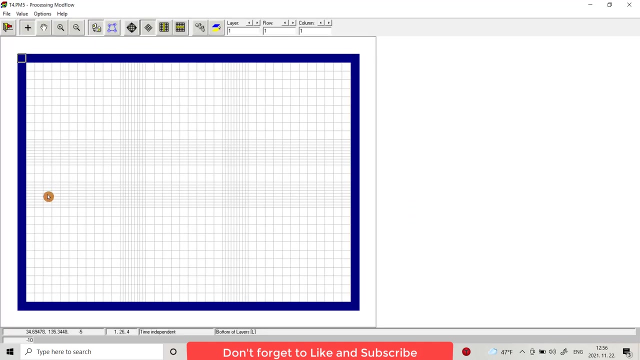 directly is a elevation for bottom and give us the elevation. you see, the elevation of the first top of the first layer is zero and the elevation for the second place will be minus 10.. yes, and bottom of layers. just show the bottom of the two layer. the bottom of the first layer is: 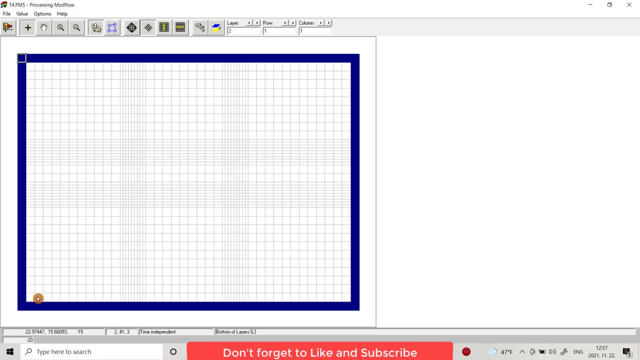 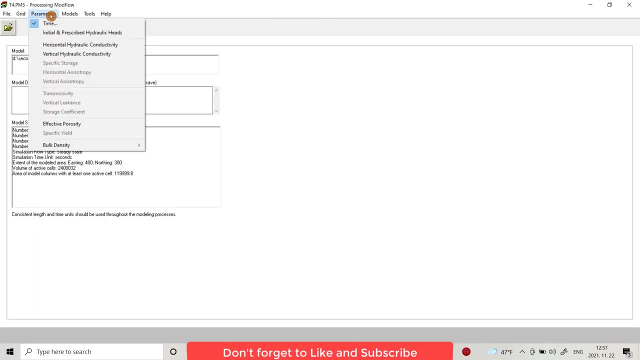 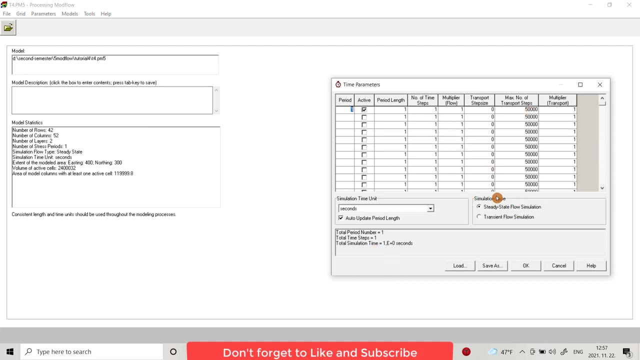 minus 10 and the bottom of the second layer. if you check, it will be minus 20.. yes, parameter time. since i use city state, you don't need this table. just we need for transient flow simulation. but this is the first one tutorial. we work with steady state flow and i choose time as days. 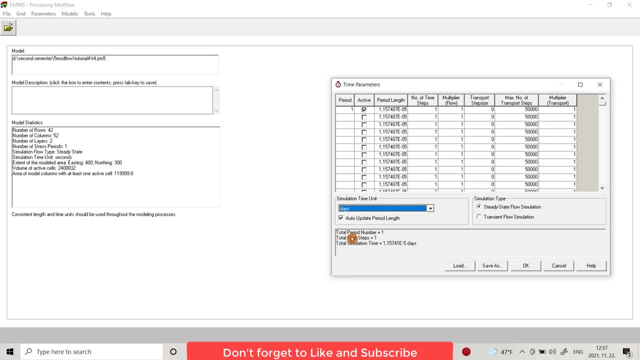 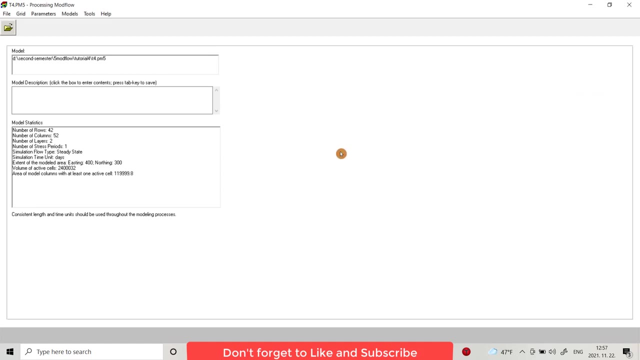 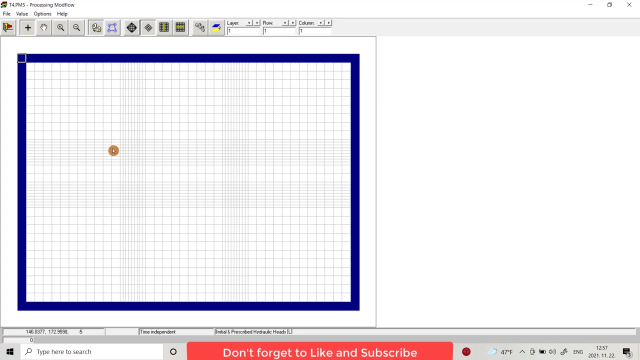 you as i told in the first one or second, a second tutorial. you should be coherent throughout the model we. i use it- length, meter and time as day. okay, initial prescribed hydraulic head. i want the hydraulic head two meter below the surface from value reset matrix changes to minus two apply. 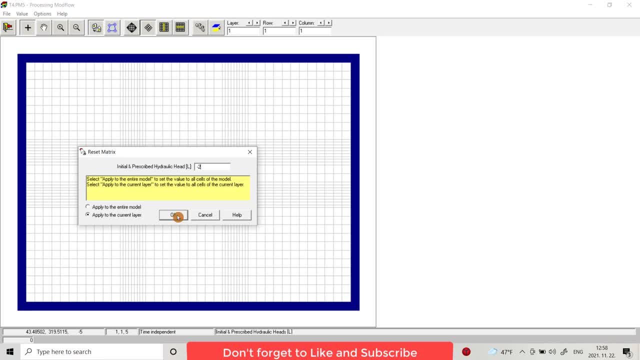 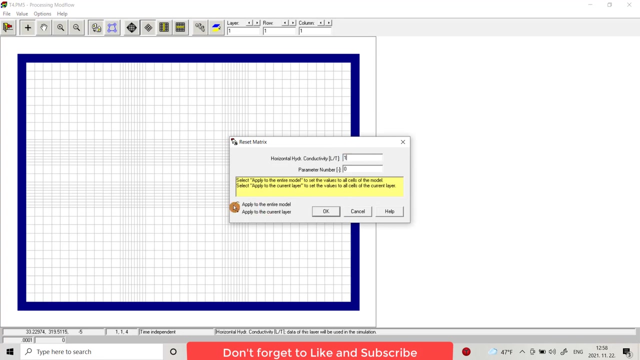 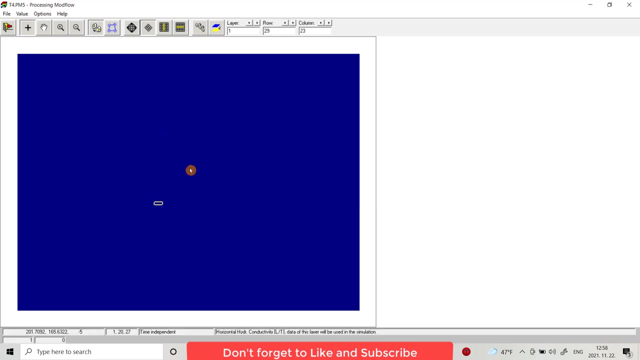 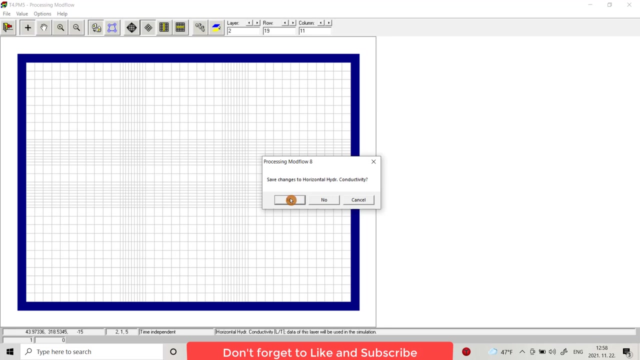 to no, the first layer, okay. yes, and horizontal hydraulic conductivity, I use, as you see here, 0.001. I choose from reset matrix one to the entire model. okay, you see one. it means all cells have hydraulic head one. if you I go to the second layer, it should be one. okay, regarding vertical hydraulic conductivity, I 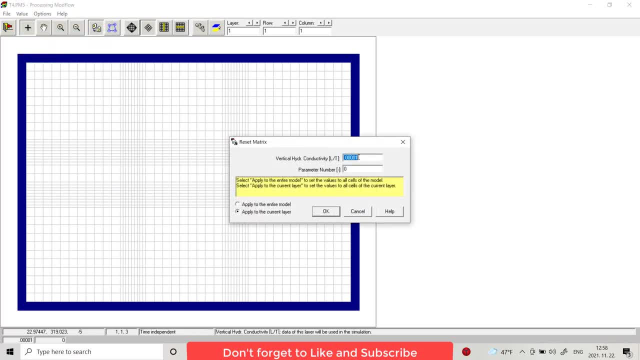 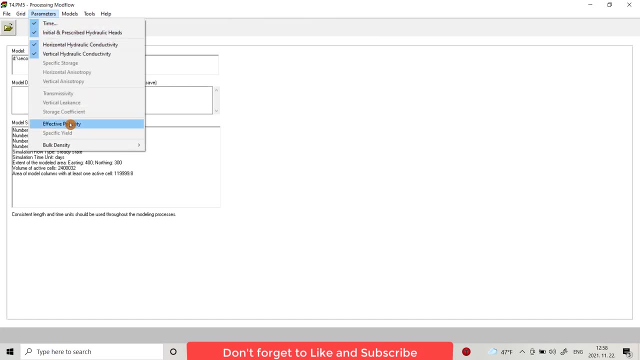 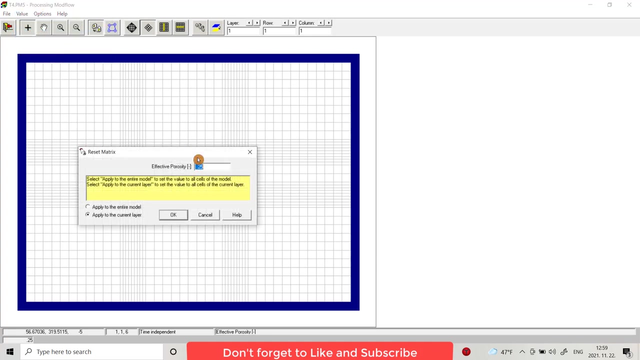 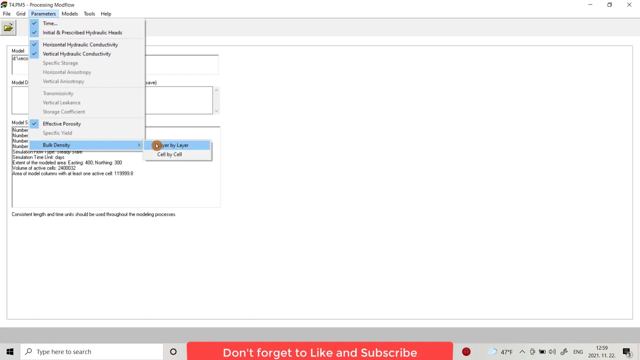 provide values: reset matrix: 0.1 to all the model. okay, we provide vertical hydraulic conductivity also, effective porosity: there is 0.25. I provide reset matrix, for example, 0.1 apply to entire model. okay, yes, the basic density, as you see, it says: 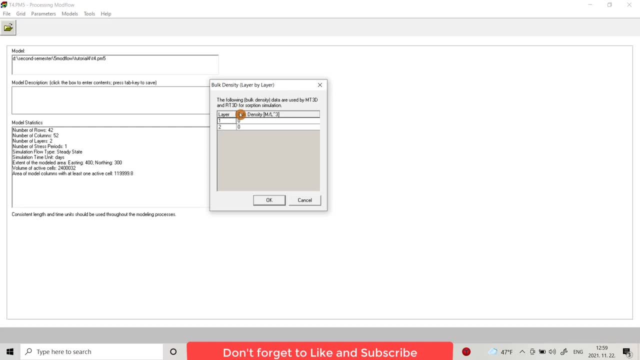 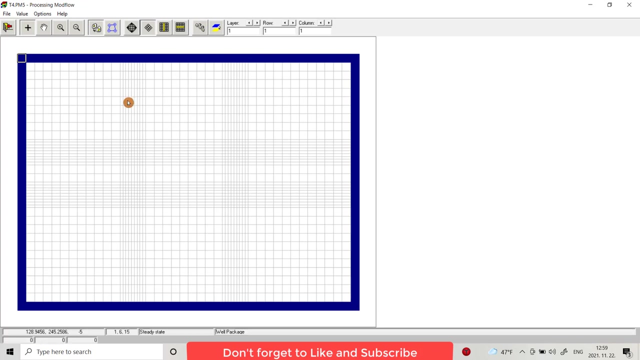 is used for code mt3d and Rt 3d, so we don't need it. okay then, from model mod flow flow package. I use wells. I provide two injection: well, in the first layer and one of the the second layer, a second layer production. well, here, right, delete just. 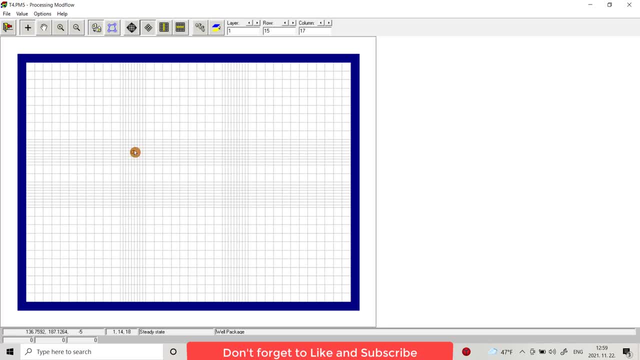 sorry, just select the cell. which cells show us? 1, 15, 70, 15, first layer, 15 column, 17 row? okay, I want to be 150, 25 liter per day. okay, you don't need this parameter number. also, you can copy. we provide the injection. well, for the first. 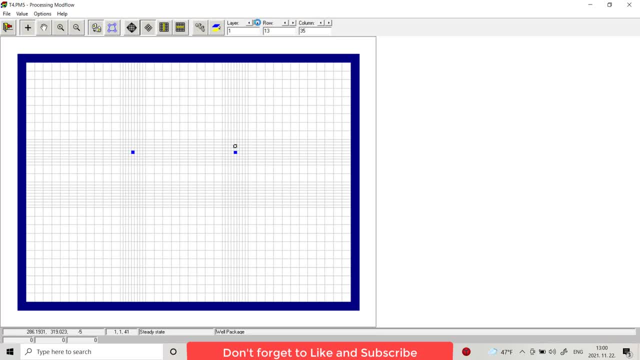 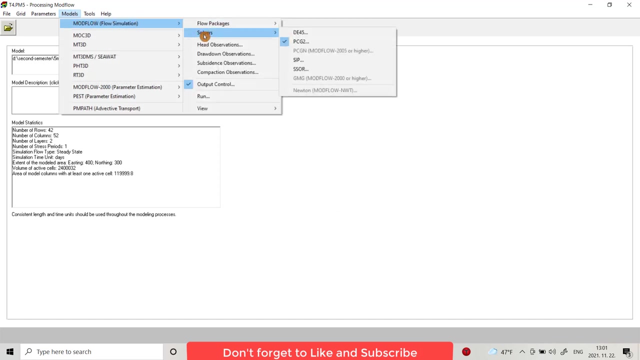 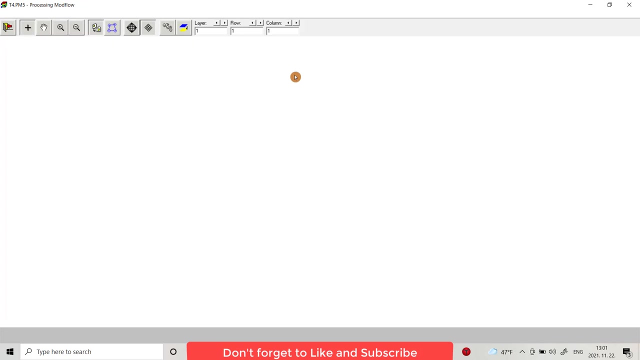 layer. regarding the second layer, I won't provide injection production. well here, okay, how much minus 50, 50 meter per meter, cube per second. okay, yes, mod flow also, I want to provide flow package drain. I want to provide recharge. for example, we have a 30 millimeter area. you. 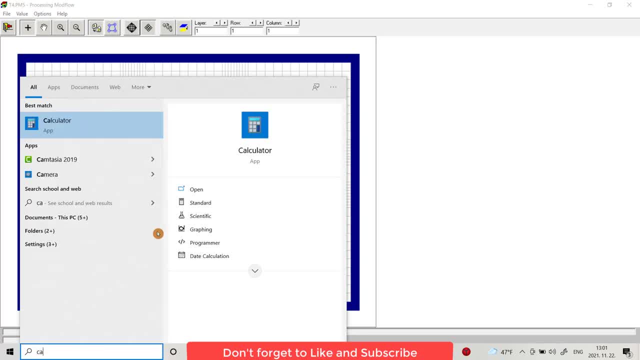 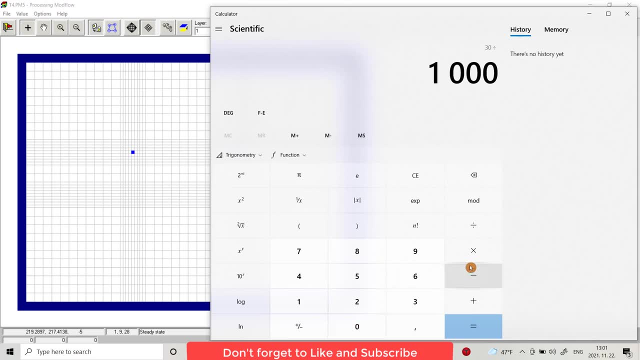 have to convert to meter per day calculator. 30 million divided by 1000, equal to 0.03. also divided by 365 days, it will be eight point two. three days. it will be eight point two, three days. it will be eight point two, three. 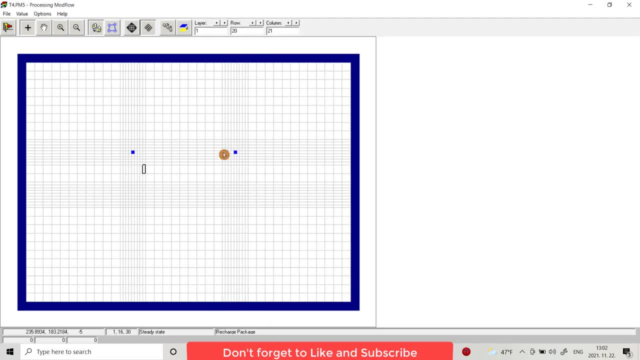 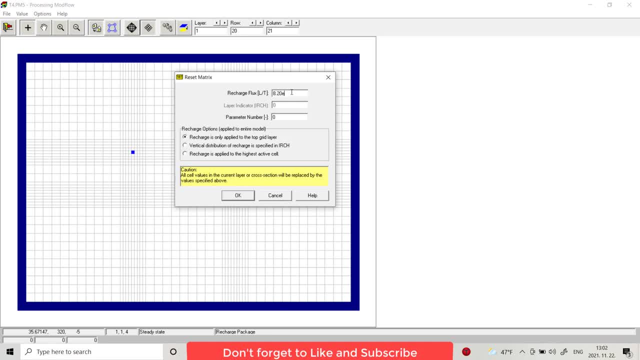 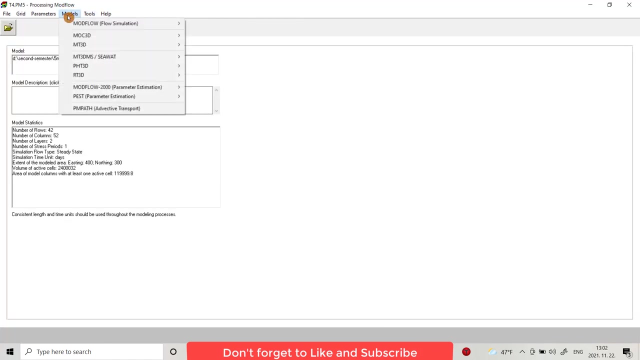 finished diesem, so we had ourselves pretty early. baby cool. began with a start with a system. already paul savory closed good cells. okay, if you see i have a recharge, it shows you that we have recharge, okay, yes, also, i won't provide from horizontal flow barrier, provide a barrier to protect a place for from. 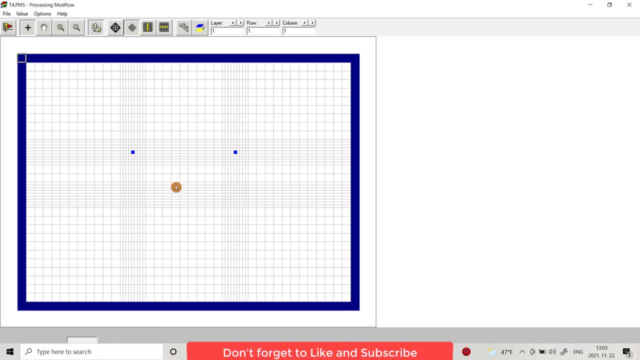 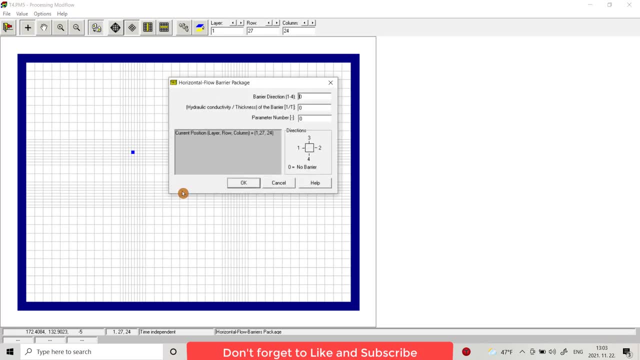 water, for example. i want to provide flow barrier here. right click it shows the direction. i provide a bentonite slurry. it is a hydraulic conductivity. you have to provide hydraulic conductivity of bentonite slurry divided by the thickness- for example, i have 10 meter and after dividing it is a. 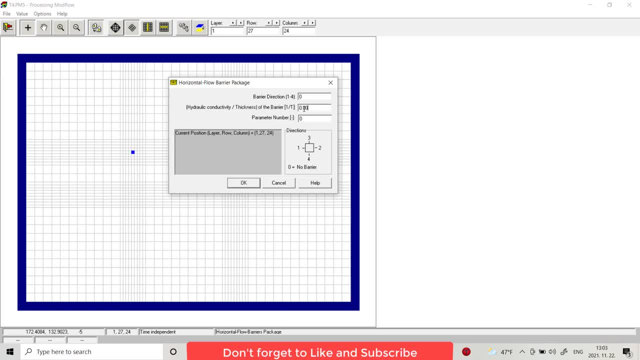 it equal 0.00. hydraulic conductivity meter per second. divided by meter per day. divided by meter, it should be 0.001. be careful: you have to divide hydraulic conductivity of the material which is a horizontal barrier is constructed. divide by the thickness of the horizontal barrier. 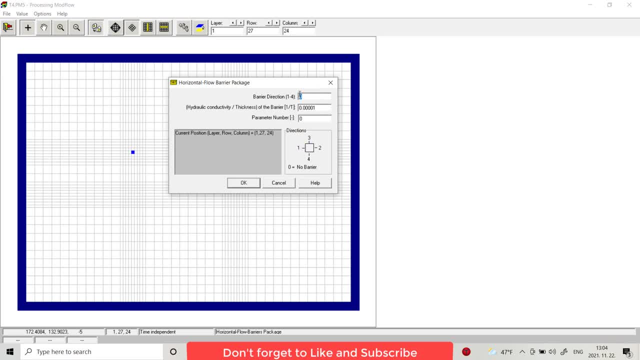 and the direction. i want to be one. go to up one, okay, yes, and copy. and by a row on your keyboard you can go up yes, and from here right click, change the direction to four. copy, copy, okay, as you see, i provide for first layer but for second layer not. so just copy, uh, just this. 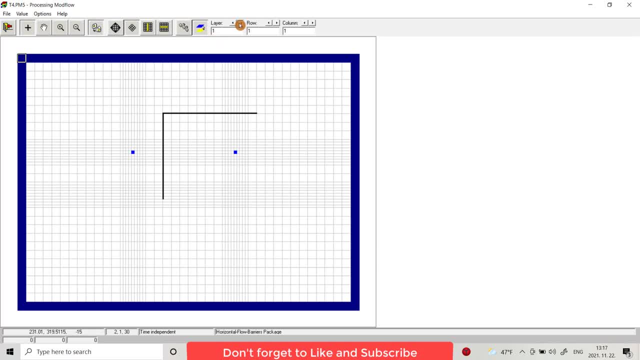 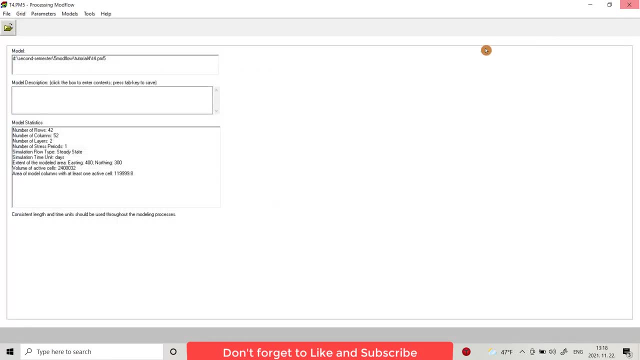 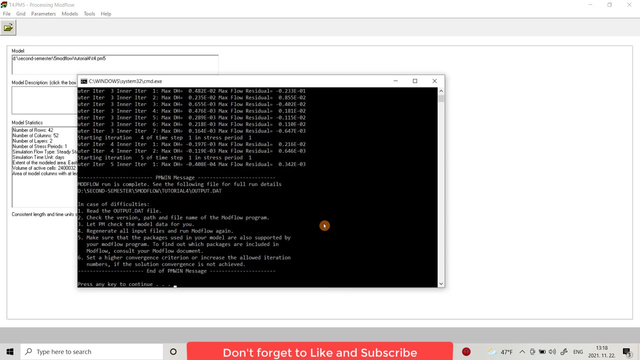 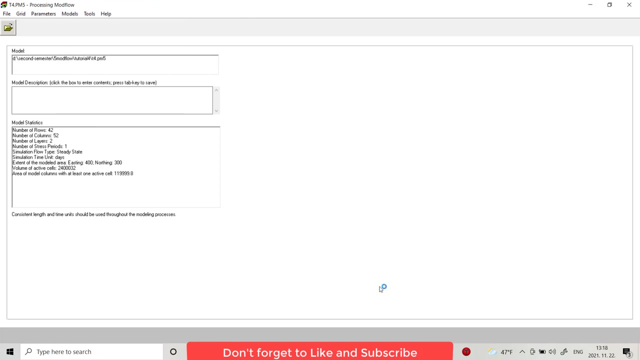 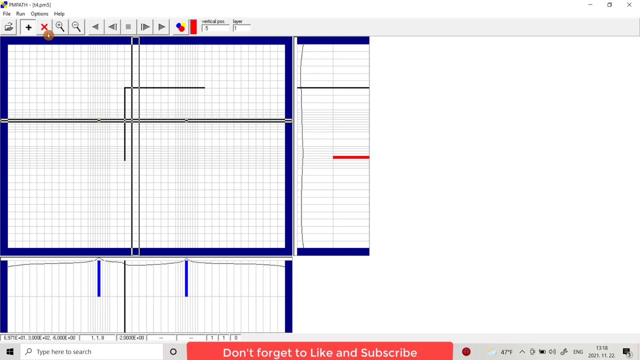 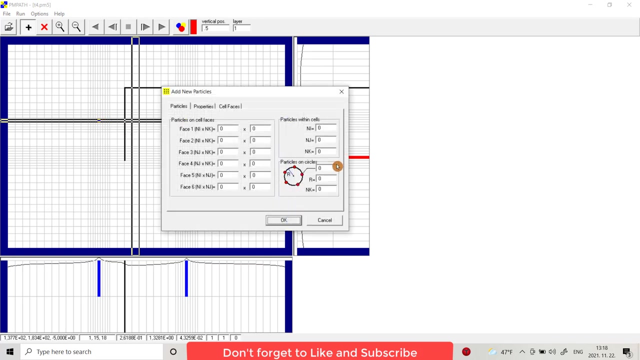 click this tab and second. there you have. now we are ready to run our model. model is mode flow: run, check, generate. okay, now i am go to model pm: pass. okay now, everything is so you just we need to bring a particles 30, 1.5, 3 layer. okay, also for: 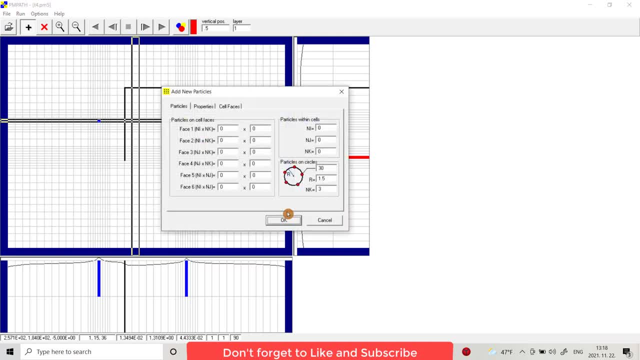 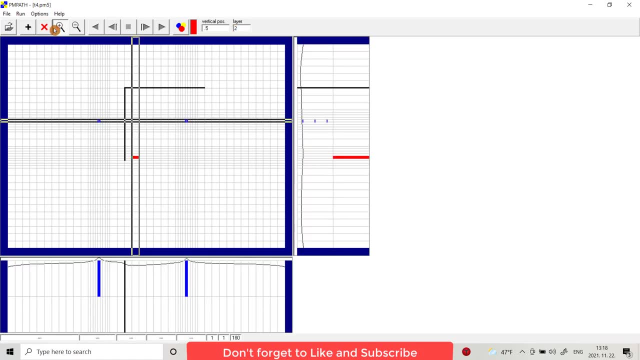 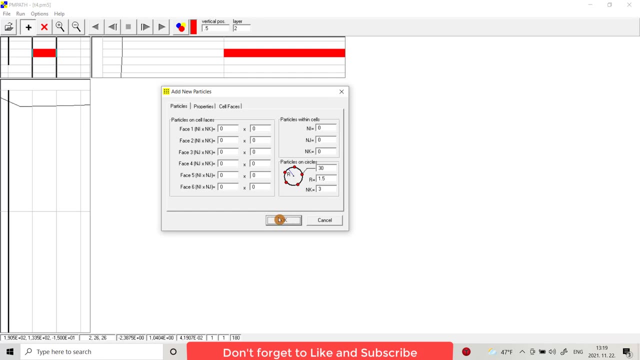 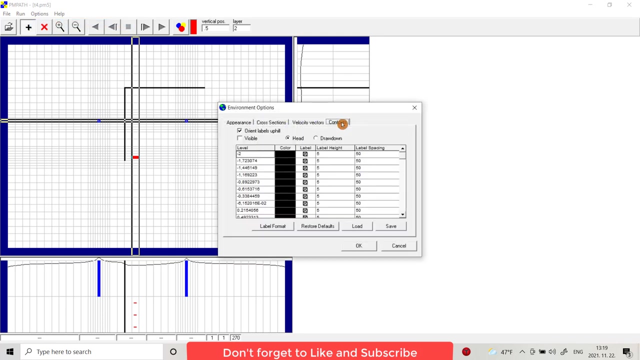 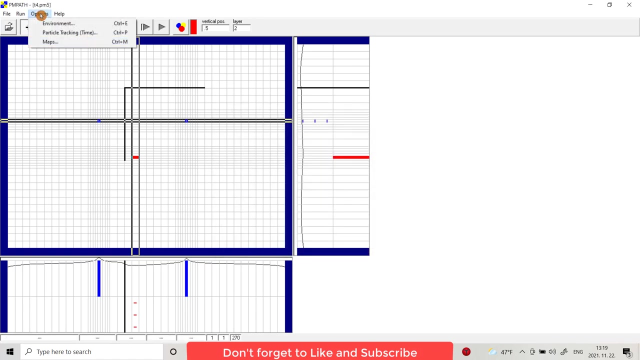 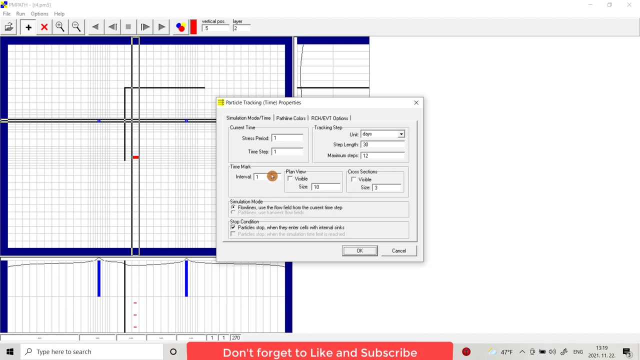 here: okay, go to second. there you can magnify here and provide particles, okay. so then from option environment- it's contours, course or a cross-section, no option. particle tracking: step length is 13, maximum step is 12 and pass line color: choose here active this one. choose for the first year blue and for second layer. 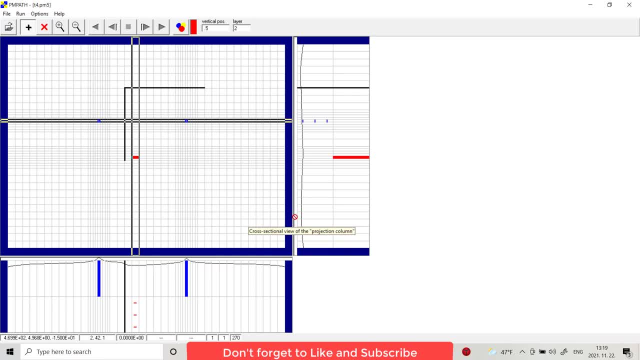 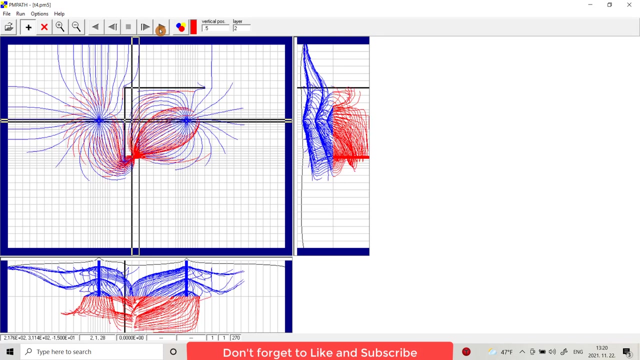 red. okay, it got forward. how the particles goes from the injection, well is, to production. well, you see, it is this one in 30 days, this one in 60 days, also. let it go and, as you see, the particles goes away from the horizontal barrier because it is impermeable. you see how it goes also. 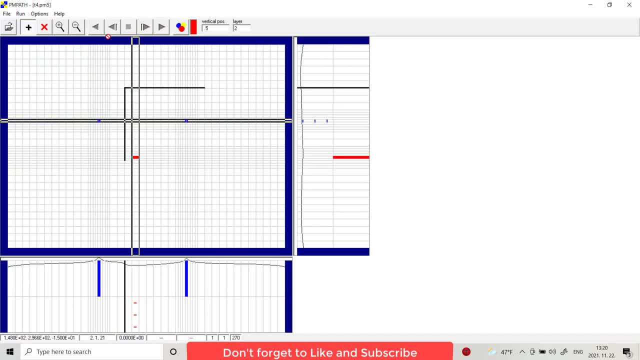 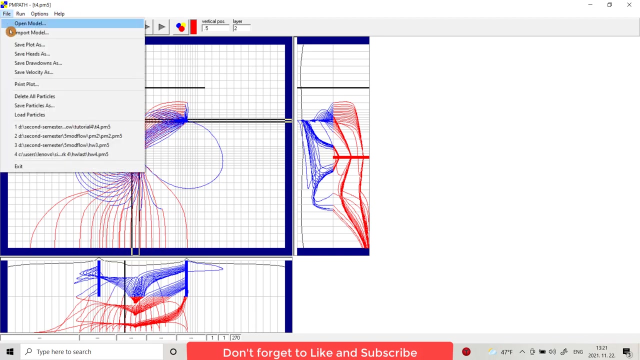 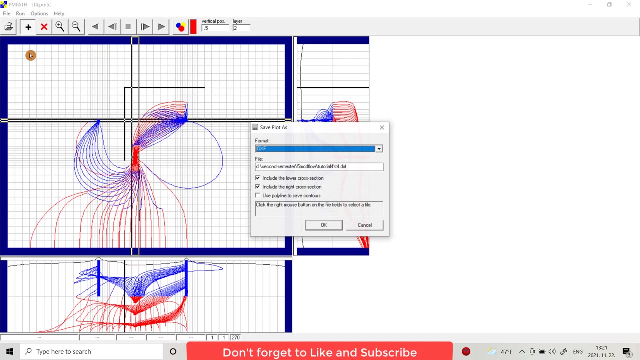 let's restart. if go, particle goes from production well to injection- well, how it should be, okay. you see also, you can save the images file. save, save plot as pxf. you can change the. you see also, you can save the images file. save save plot as pxf. you can change the. 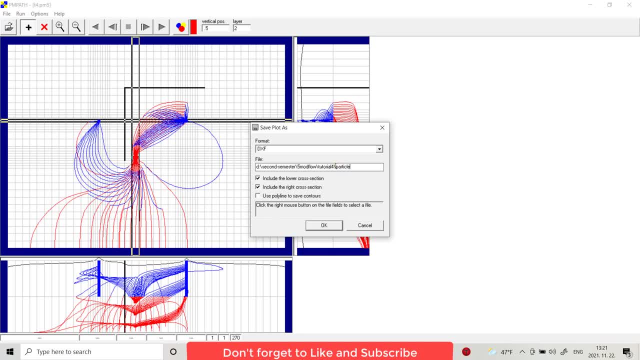 name article production injection mean from production to injection. well, you can save it. you can save as dxf file and the xf file. okay, you can use it with a autocad. that's it to save the images file. save plot as pxf file. save plot as pxf file. save plot as pxf file. save plot from pxf file. save plot.